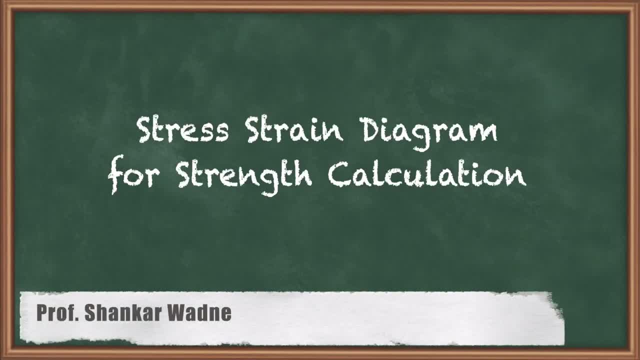 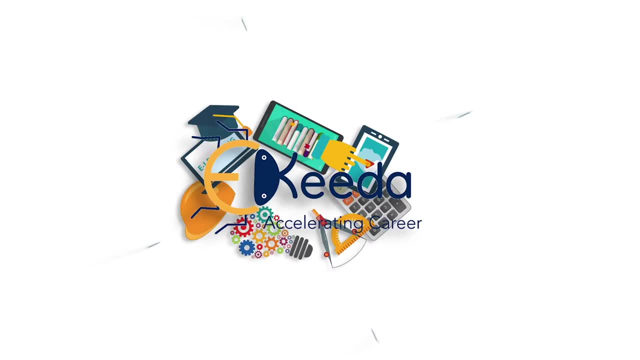 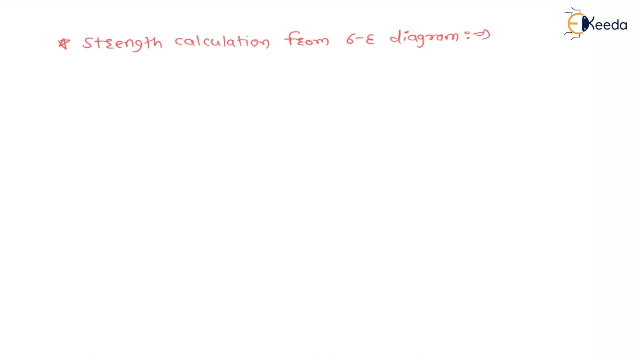 Hello, my dear students, In this lecture we will see how to calculate strength point with the help of stress-strain diagram. Now, while calculating strength, we have to calculate strength for ductile material as well as brittle material. We have to calculate for ductile as well as for brittle material. 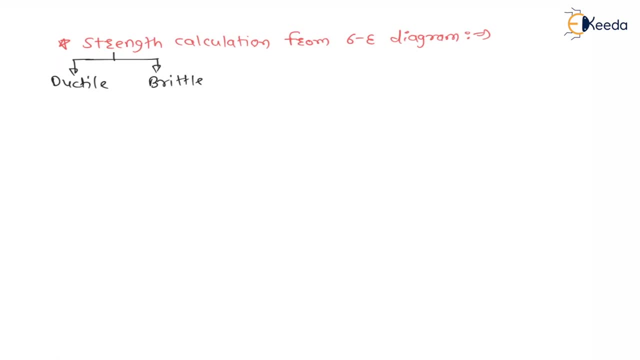 Now. hence we will see stress-strain diagram for both ductile as well as brittle material and how to find strength point with the help of this stress-strain diagram. Now, if I see ductile material first, if I see ductile material, let us say steel, Steel is a ductile material. 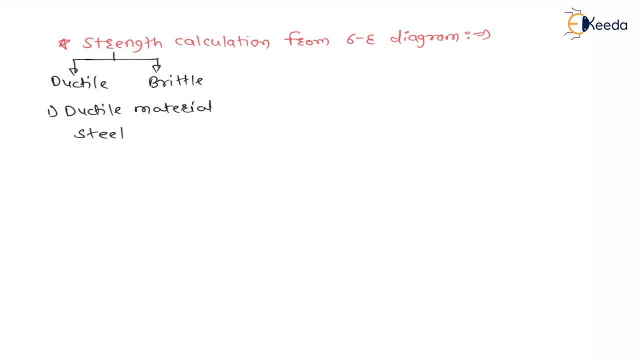 If I consider steel, steel is a ductile material. Now, this steel is nothing but alloy of iron and carbon. It is a Fe plus C Now in iron. in iron, if this carbon percentage percentage of carbon is 0 to 0.25. 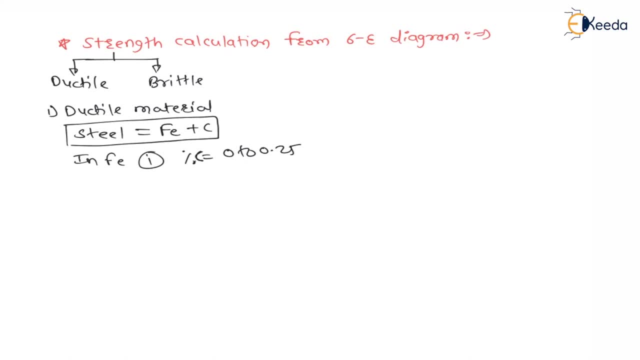 If the percentage of carbon in iron is 0 to 0.25, then it is called low carbon steel, Then it is called low carbon steel Right, And in iron if this percentage of carbon percentage of carbon becomes 0.25 to 0.45.. 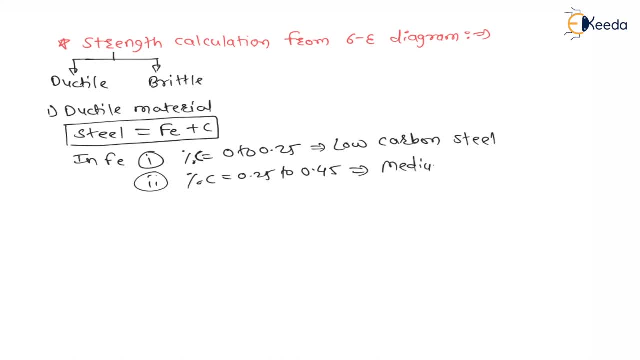 Then it is called medium carbon steel, Then it is called medium carbon steel. And in iron, if this carbon percentage percentage of carbon becomes 0.45 to 2.11,, 2.11,, it is called high carbon steel. 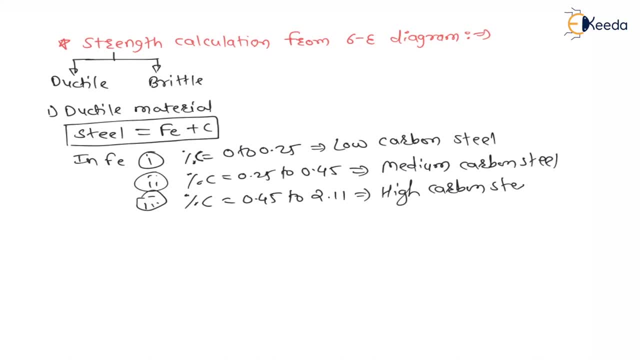